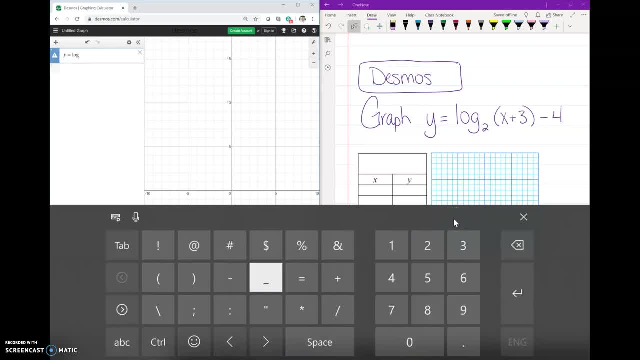 Shift dash gets you that underscore. But you want to use that underscore and that lowers it down into the base And then you can type in that it's a base of two And then you use your right arrow to get out of the base. 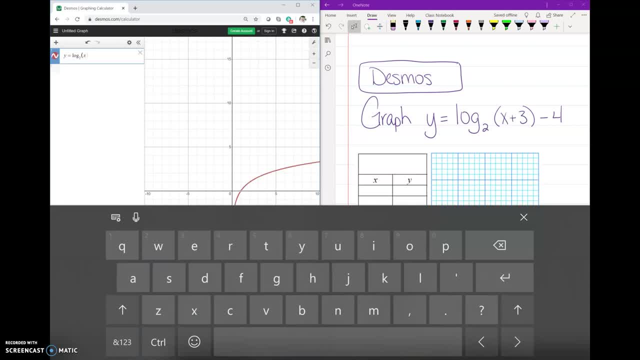 Parentheses: X plus three. The way that this does my keyboard is kind of annoying, but oh well, Right arrow, Get out of the parentheses and then type in minus four, And minus is just using the dash Or your minus button on your keypad. 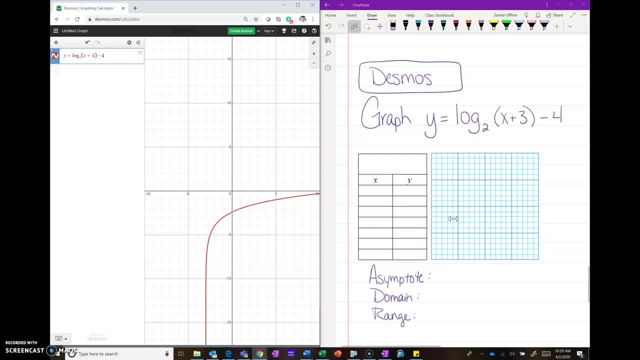 And that graphs it for you. Now this shows you the graph, and the nice thing about Desmos is that you can physically move this graph around and look at it, Which is something that you really can't do on the graphing calculators. so I do love Desmos for that. 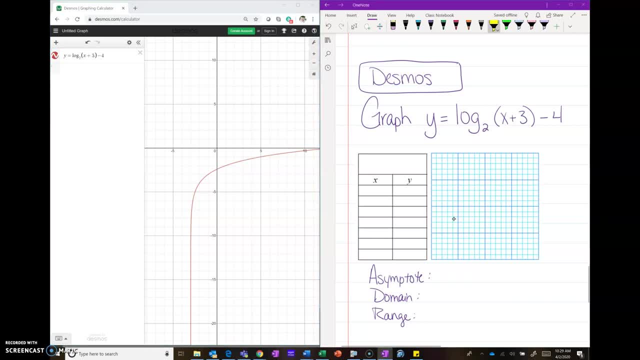 You can see that the asymptote is at negative three And you can also You'll see that in the equation. The X plus three tells us that our asymptote is going to be at negative three. That moved the graph left three. So if I've got my Y axis straight down the middle, imagine that that's straight. 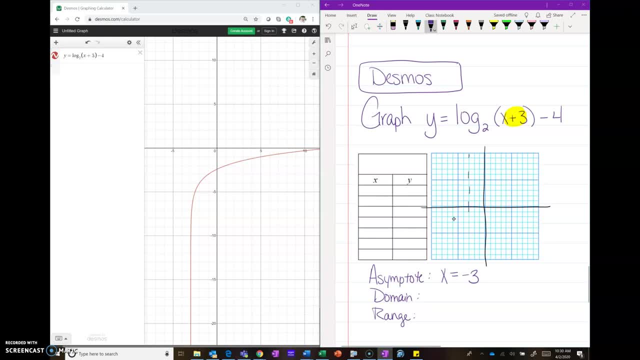 Your asymptote is at negative three. You should draw in a dashed line at negative three so that when you draw in your graph you aren't tempted to cross that line. Your domain is tied to your domain or to your asymptote. So our domain is X is greater than negative three, because this graph is on the right side of that asymptote. 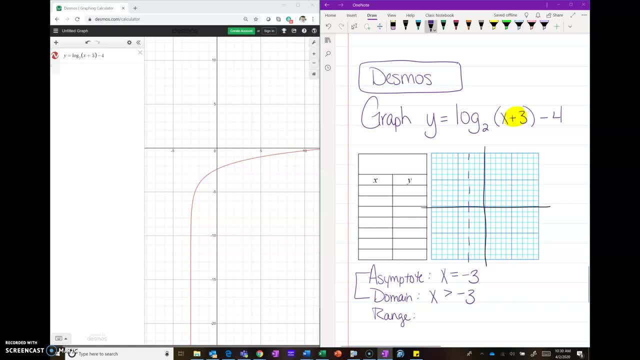 To get points in Desmos. this is where it's a little bit tricky. You need to click the little wheel, the settings wheel, which says edit list, And then grab the thing that says that looks like a table and it says convert to table. 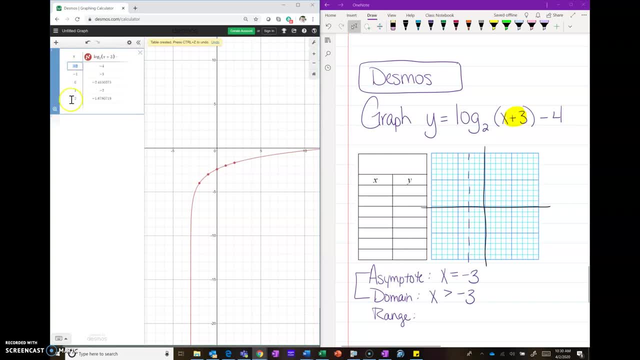 This converts this equation into a table and the points that are shown in the table Are shown on the graph, which is kind of helpful. So on this one I can see the points that I definitely want to use. I want to use negative two, negative four, negative one, negative three and one negative two. 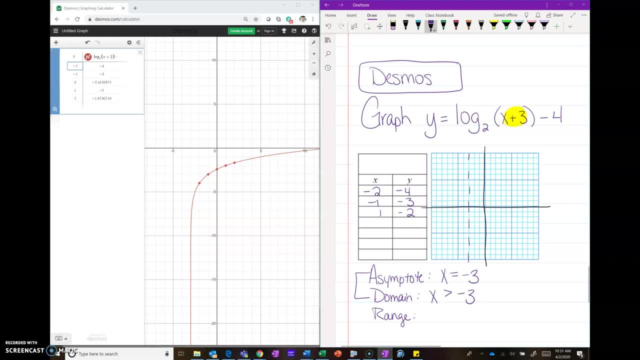 But say I didn't have any good points. If I wanted some different points, you can go right down below this table and just start typing things in, So I could type in: three, enter, four, enter. I think it actually starts just doing that for you. 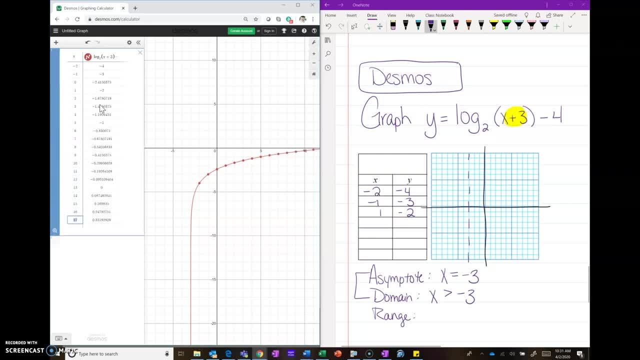 So five, six, You can just keep hitting enter and you can get a whole bunch more points on that table. So you have an endless number of points. And if you wanted to say, oh, I don't know what is what, if I wanted to graph the point with an X value of negative 2.5?? 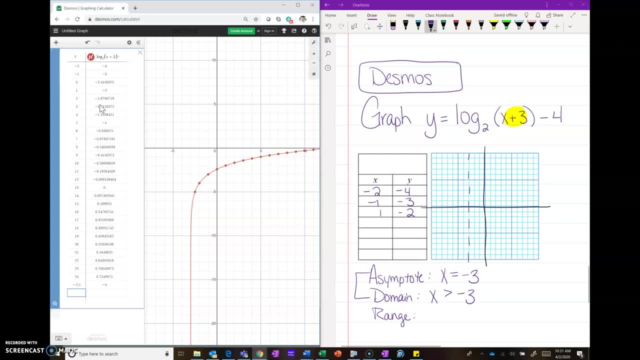 It would tell you that that was negative five. So negative 2.5, negative five. that would give us a point that we never could get on our graphing calculator. So that's kind of cool. All right, We plot these points: negative two. negative four. negative one: negative three: one, negative two. 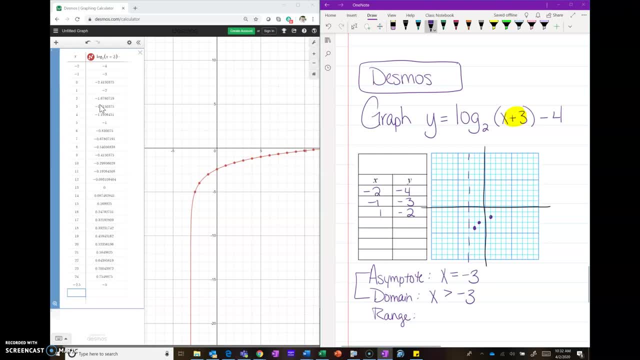 If we wanted to, we could plot that point: negative 2.5, negative five. That would allow us to get even closer to that asymptote. On the right side, this graph is going to continue off and you could even look and see how. 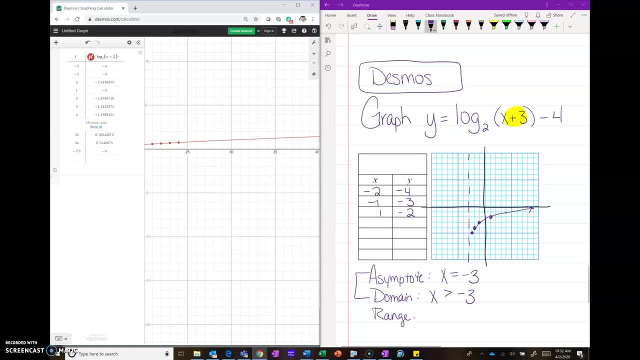 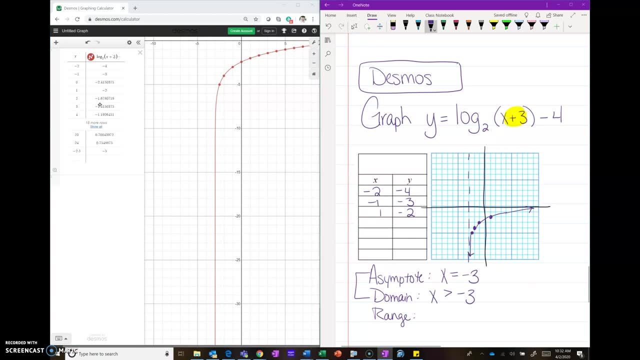 see how it continues to go up and up and up, just very, very slowly. And on the left side it gets very, very close to that asymptote, but it never crosses it. Our range is all real numbers. If you wanted to then graph a different one, you could just hit this little X. 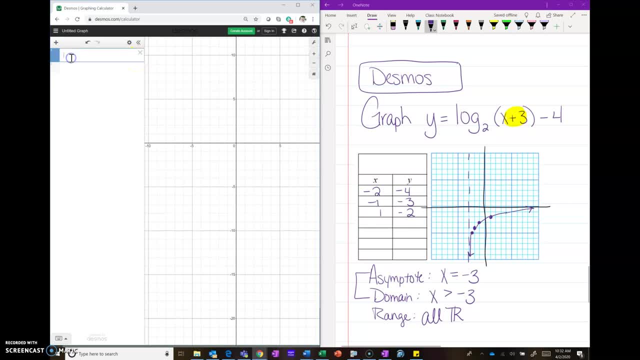 and it clears it out And now you can type your next equation in. The other thing to notice is there is a keypad at the bottom of Desmos, So if you don't know how to type something, you can type it in here. 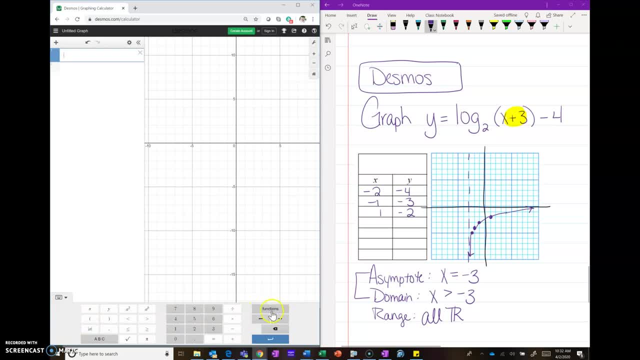 If you don't know how to type something in, you can hit this little keypad and then you can go to functions. And it's kind of weird, like this, first function list is trig. We don't want any of that. We don't really want stats. 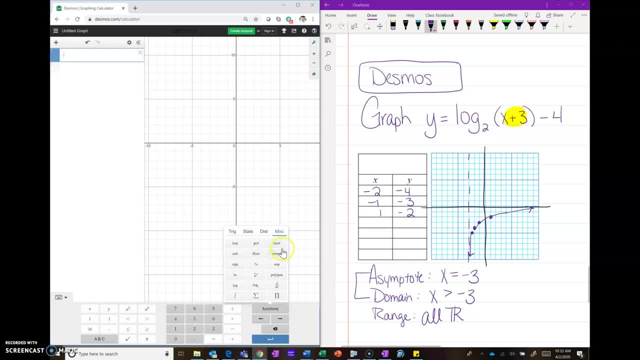 We're not talking about distance Miscellaneous- Inside miscellaneous. there is log. They even have a button specifically for log base and for ln. So if you wanted to graph y equals, type in y equals, then you could go into the keypad, go to. 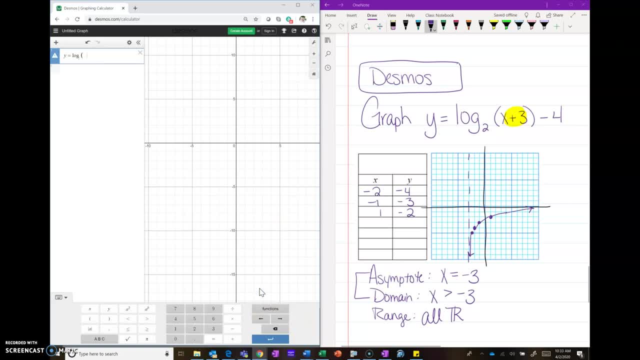 functions miscellaneous and you could click in log base and it puts that template in for you so that you could fill in log base 2 of x plus 3 minus 4.. So there's a couple different ways that you can enter things in Desmos.